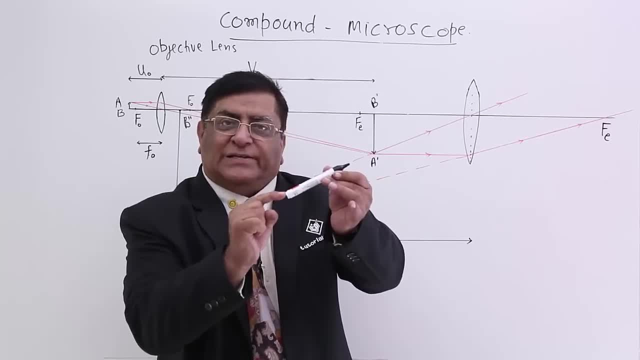 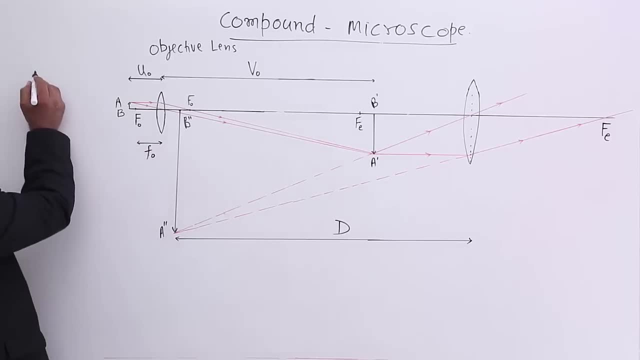 the one lens where we will place the object is known as objective lens. This is that lens. What is the specialty of objective lens? This has got small focal length. Okay, It has got small aperture, because for small focal length it is necessary that aperture. 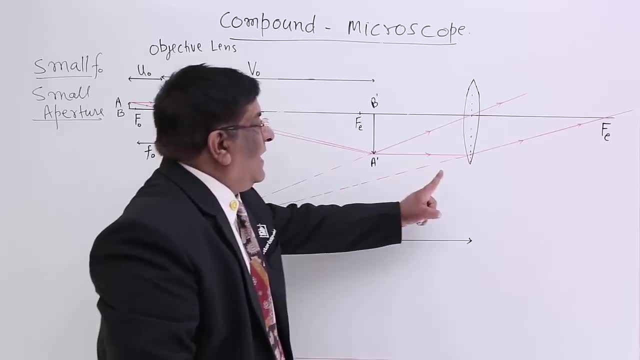 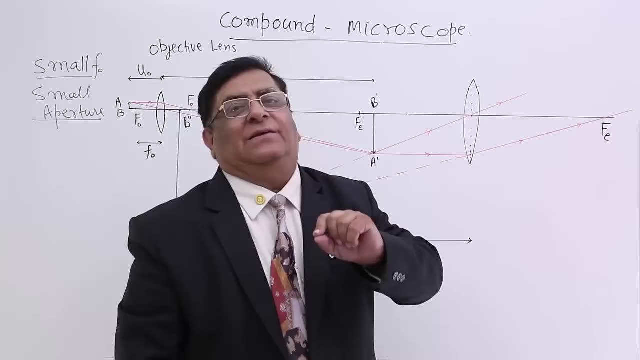 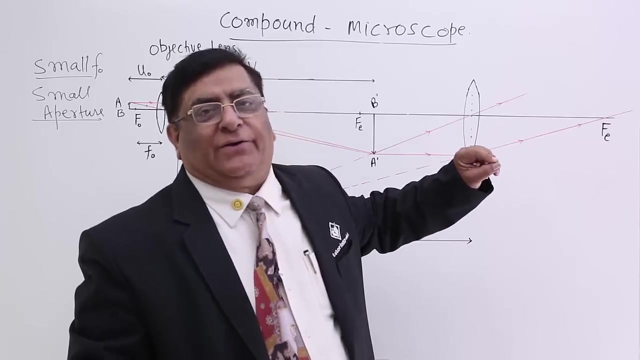 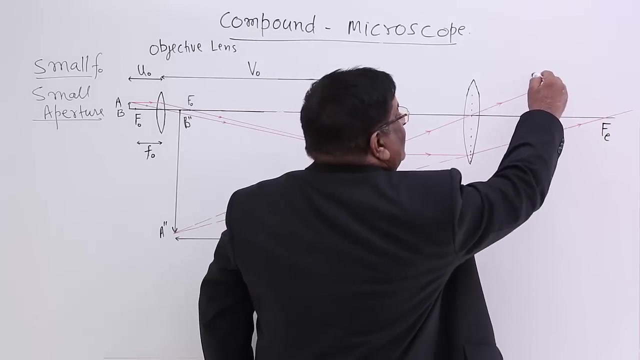 is small. Okay, Then we have another lens here. This is again a spherical lens, a convex lens, and it acts similar to a simple microscope. It has the same job, simple microscope job. So we have two lenses, We keep it near the eyes and we observe any object from this side. 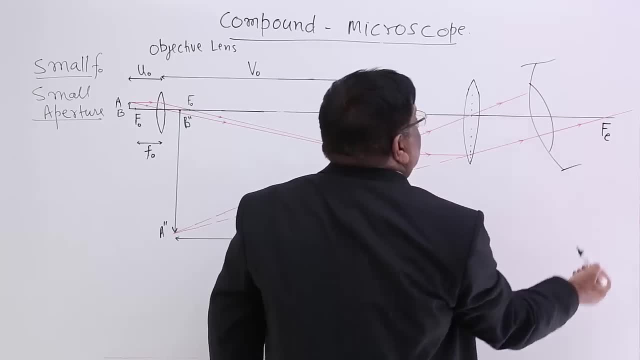 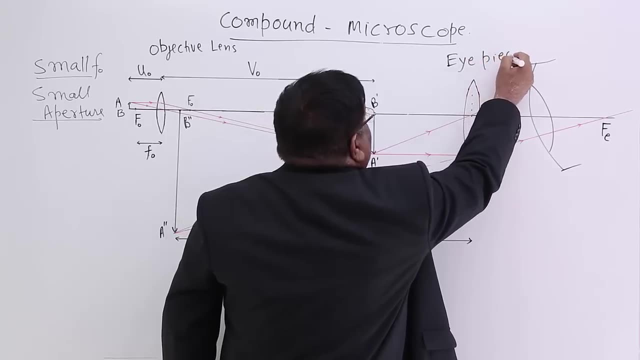 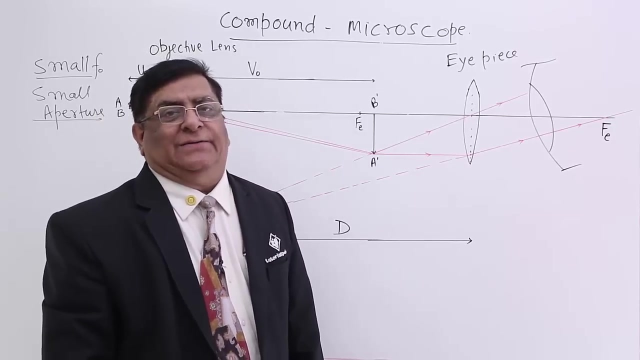 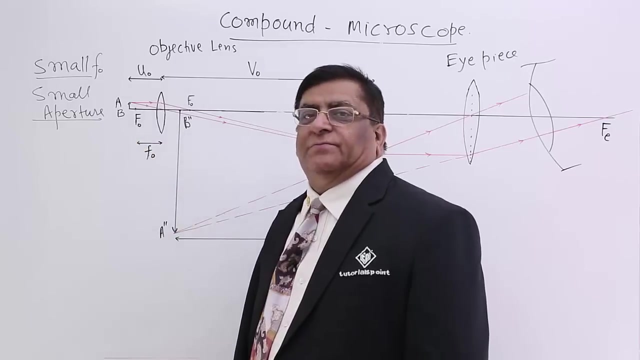 This is our eyes, So this is close to the eye. We call it eyepiece, Eyepiece or eye lens. Okay, Now how do we do the setting? See, the object is placed so that the object is slightly outside the focus. Remember, these are all small questions and very important. 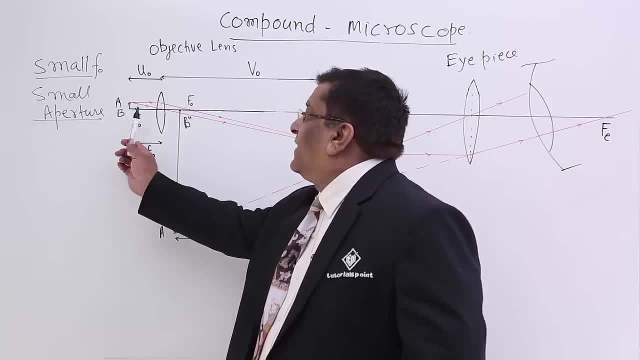 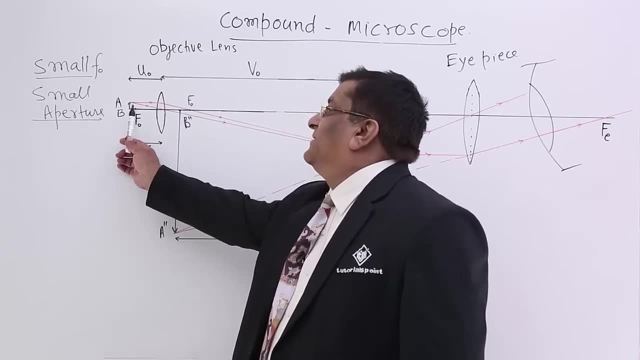 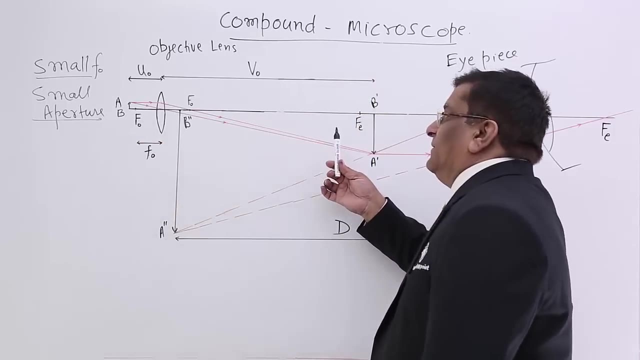 questions. Where should we place the object? Slightly outside the focus, Okay, But not very much outside. When we place it here, where will be the image formed? Answer: image will be formed on the other side, That is, on this side, One ray which comes parallel. 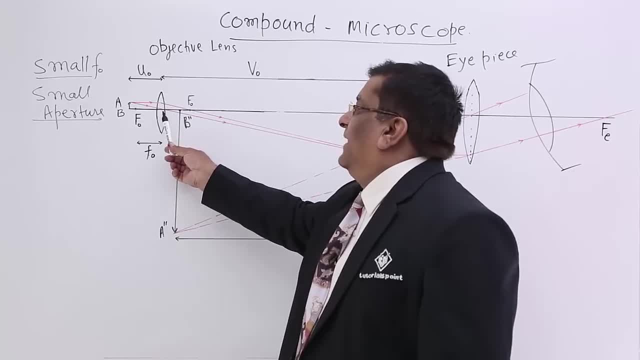 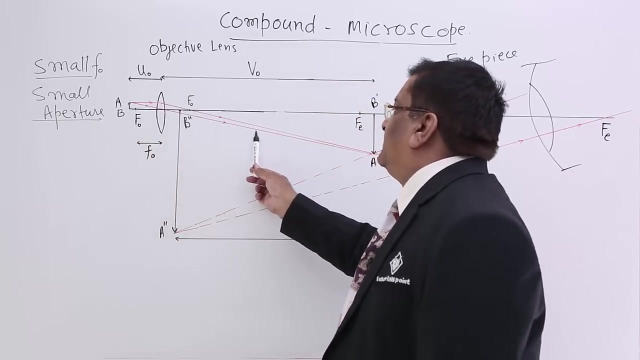 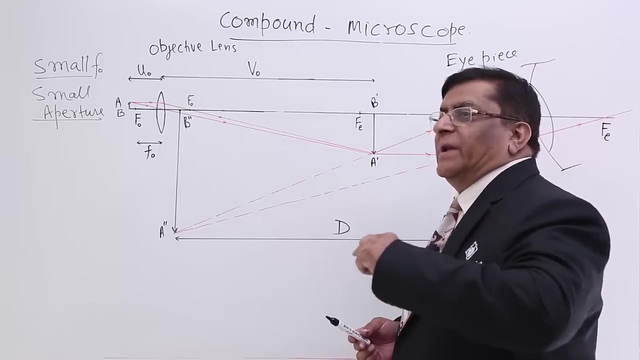 will go through focus of this lens. Lens has got two focus, one on this side, one on this side. So the parallel ray will pass through focus. Another ray, which is passing through optical centre, will go straight and both are converging. converging meet at a point actually. 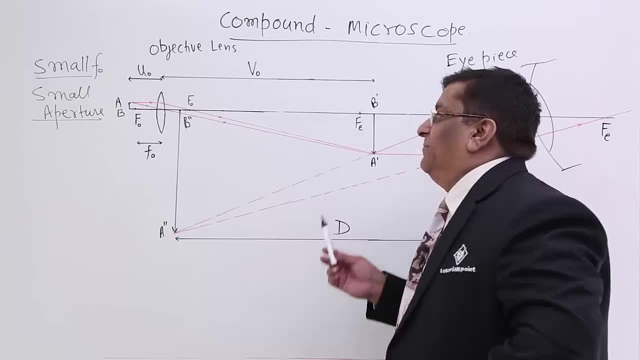 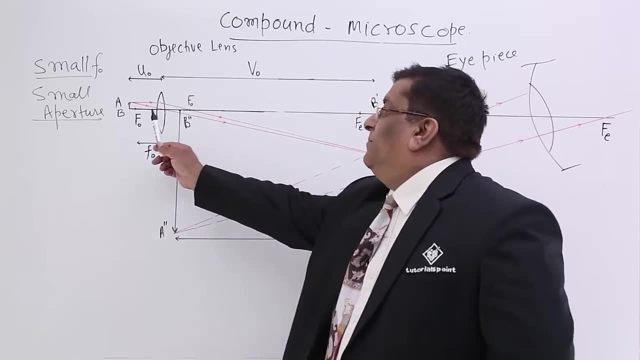 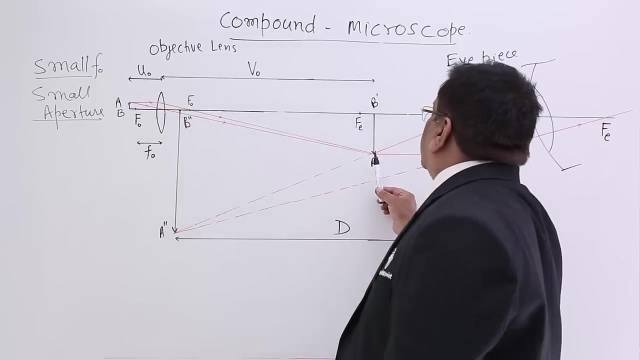 When they meet at a point, actually they make a real image. Real image of what? Real image of A? Real image of A. that is A dash. The image of B will be made on principal axis and perpendicular to the principal axis. So we make a perpendicular here. So A, B makes an. 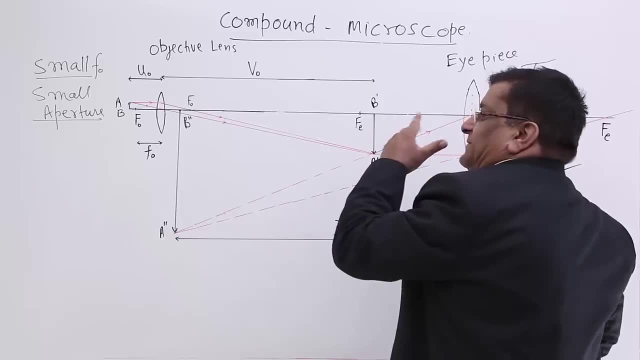 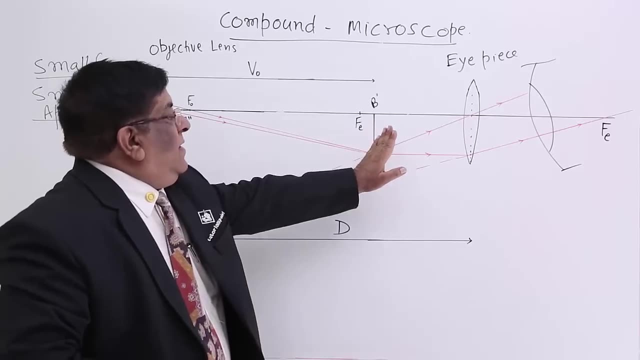 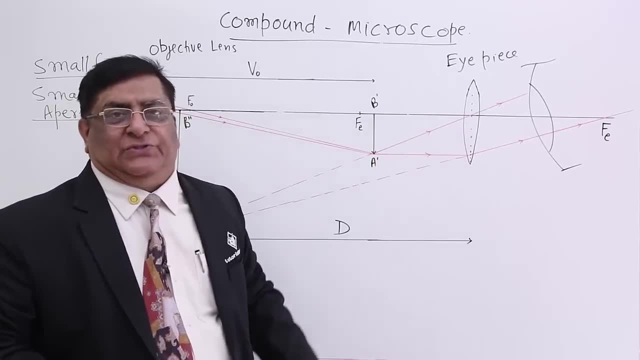 Okay, Okay, Okay, Okay, Okay, Okay. vrai voilà, Right, Okay, Okay, Okay, Okay Okay. Transrestrial is fine to the eye, but the find point of the lens is V. If one object is visible to the자 to your left, its workers will demanding that which. 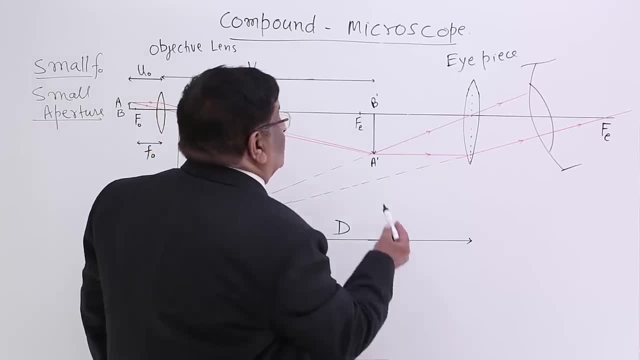 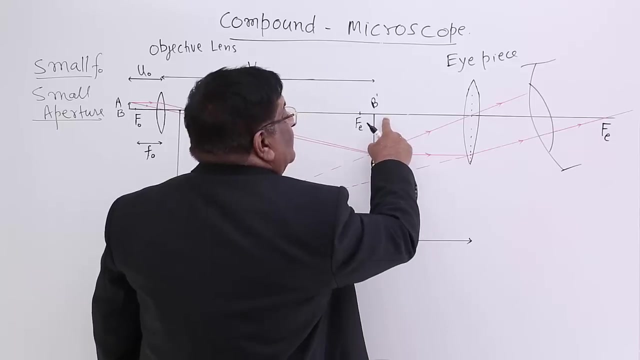 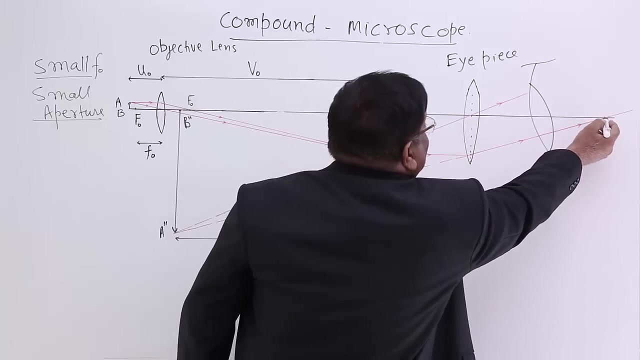 one, and if its object line is in the middle우�, então cogn spiritual point of view will need to be in middle, Correct ire times. From celestial plane goes out A Yes, Yes Does not change Sek. Yes, go through. focus of this lens here. this lens again has to focus. one is here, one is here. 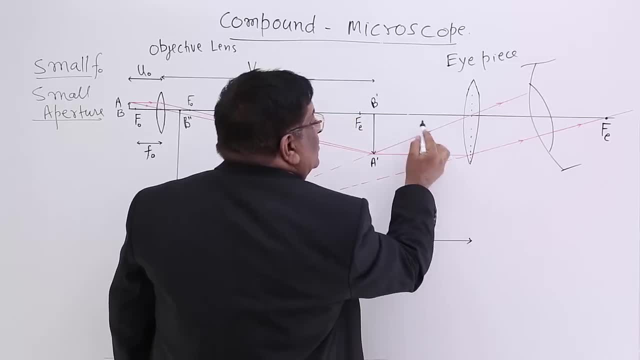 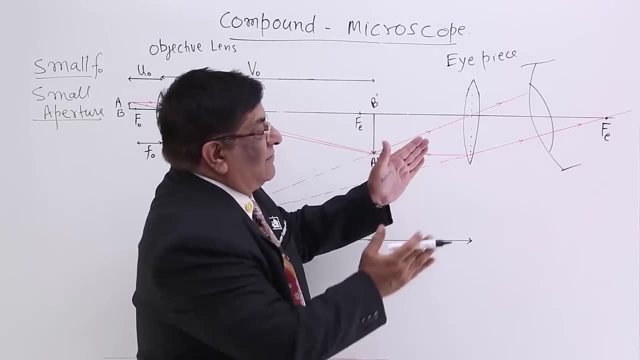 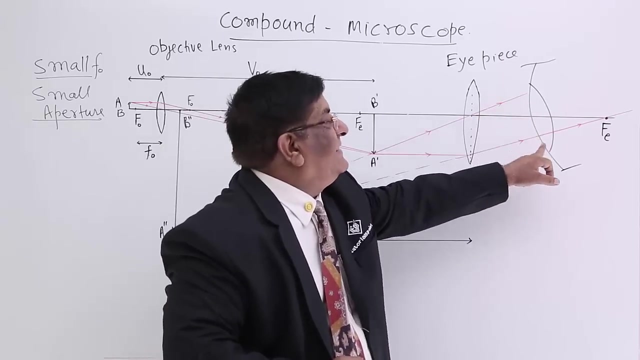 same distance. so this will pass through the parallel, one will turn and pass through focal length here. now these two are diverging, they don't meet, so they don't form any image on this side. when I put my eyes here I see one ray is coming from this direction and other. 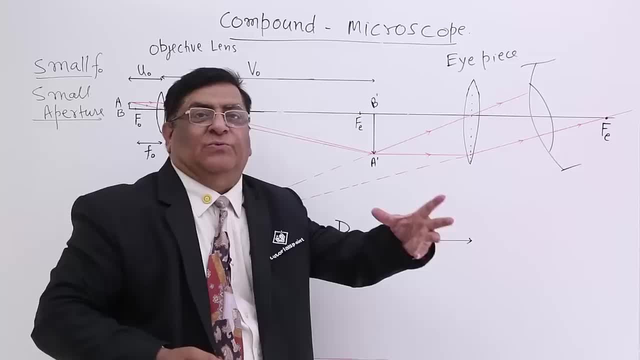 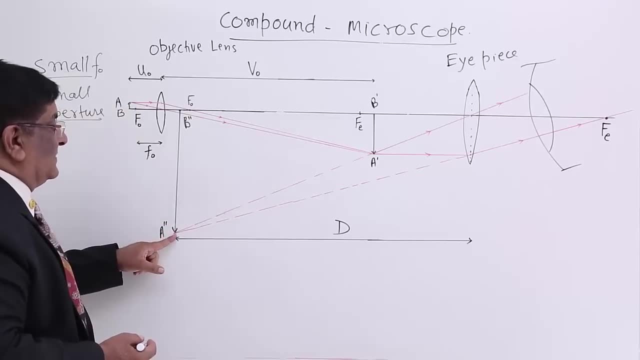 is coming from this direction. so what do I perceive? where is the image where the two rays meet, and they two meet at this place? here I see image of A dash- I call it A double dash- and then draw a perpendicular because B dash will form its image on the principle. 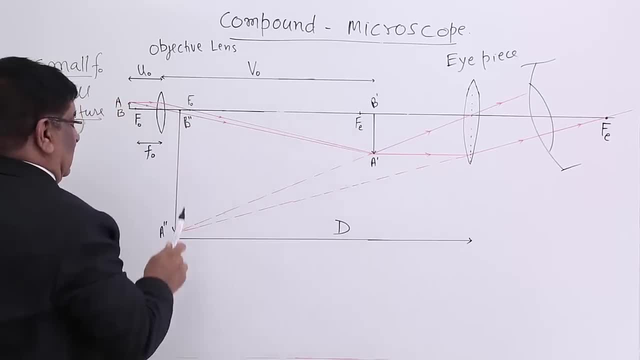 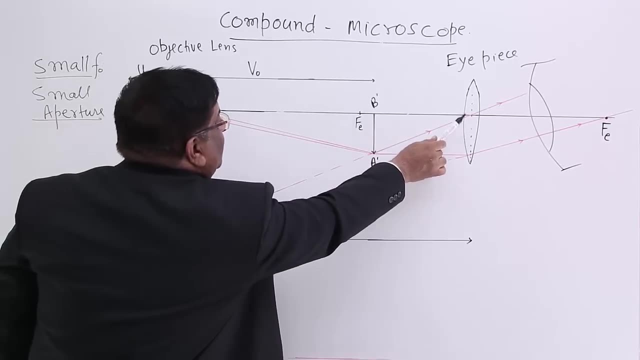 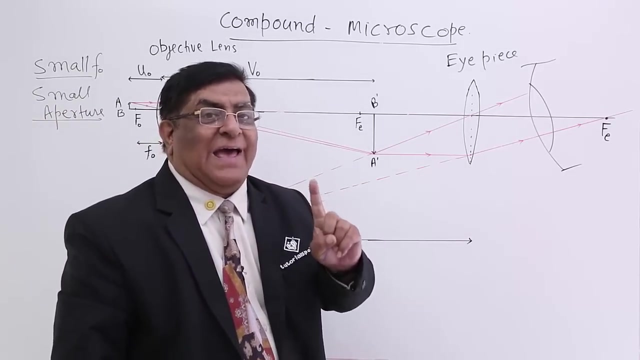 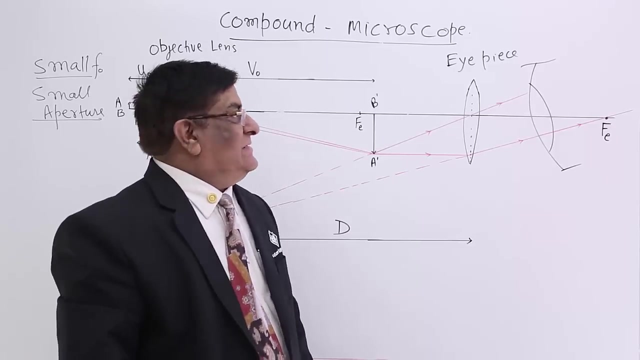 and at right angle here. So A double dash, B double dash is the image of A dash, B dash as formed by eyepiece. This eyepiece I have taken care to set as simple microscope for distinct vision. How do we place that? Answer is: the focal length is outside and this object 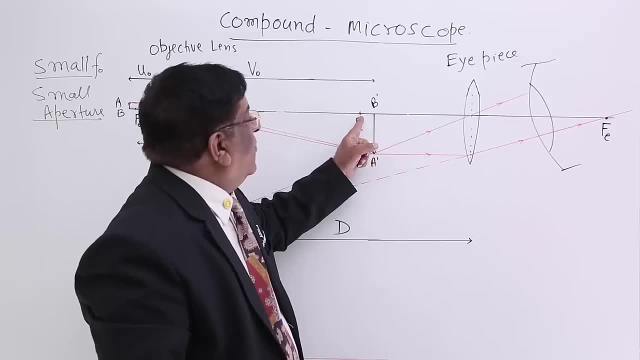 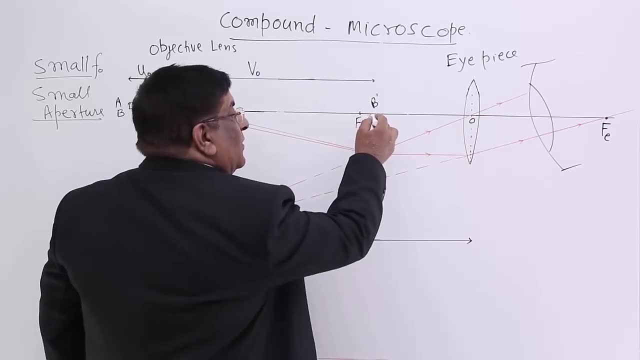 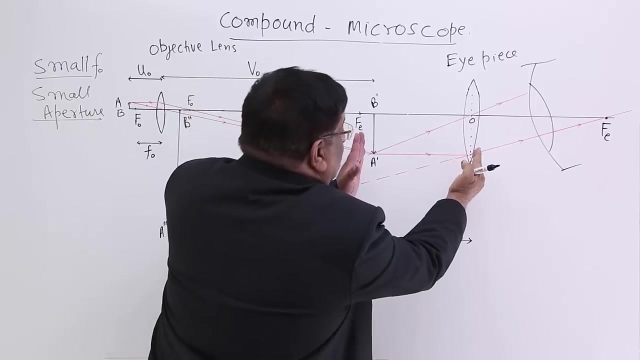 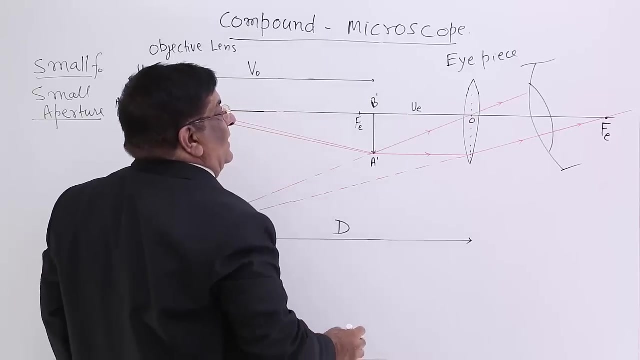 made is kept inside focus and optical centre. That is what we studied when we were studying simple microscope. The object is between focus and optical centre. Then by adjustment of this U, this distance, this is what U for eyepiece. So this distance we adjust so that 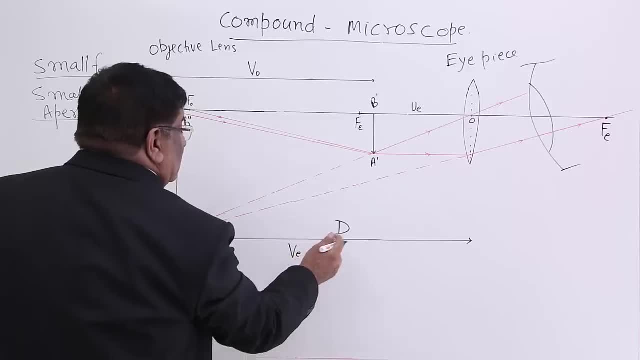 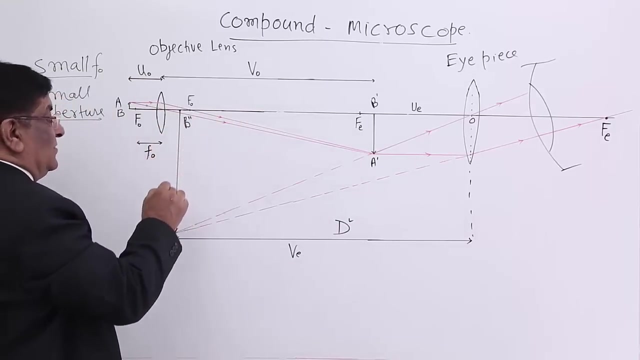 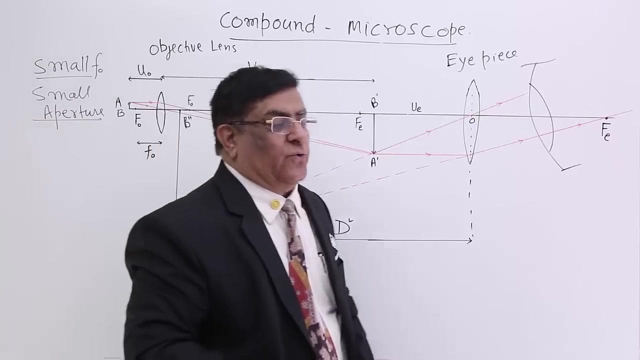 this V for eyepiece. This also keeps on increasing, decreasing, and we set it in such a way that this V become equal to distinct vision. If this is equal to distinct vision, then I am able to see this image most clearly, So I set it that way. This is how a microscope is set Now. 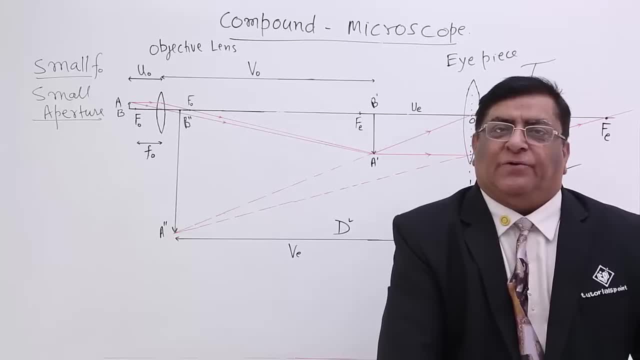 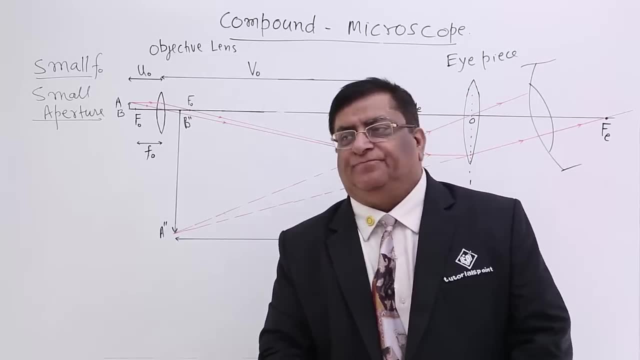 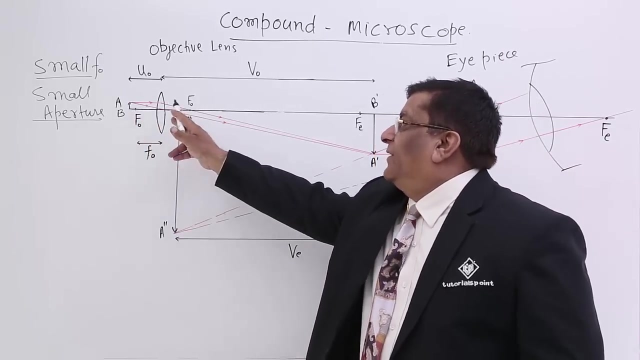 this is setting for distinct vision. There are two types of setting: One for distinct vision and one for parallel rays. So this is setting for distinct vision. Okay, And now I see A double dash, B double dash. finally, we all see this object. how large. 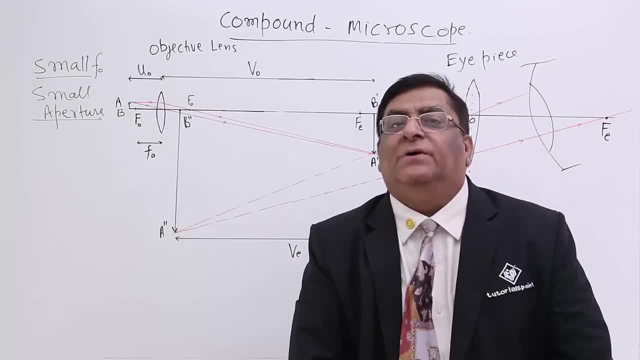 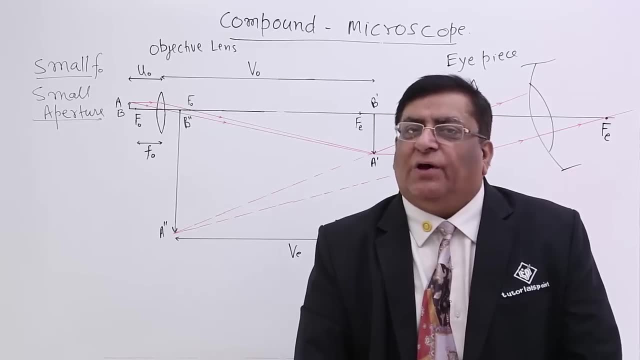 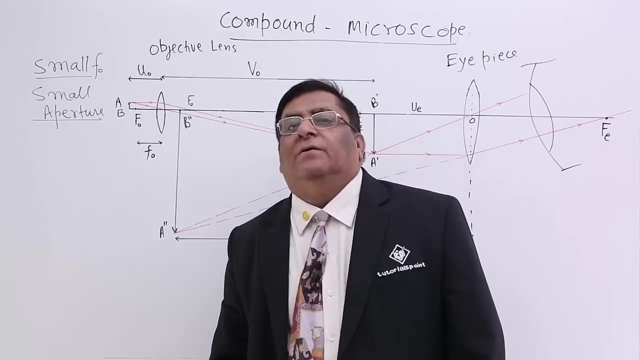 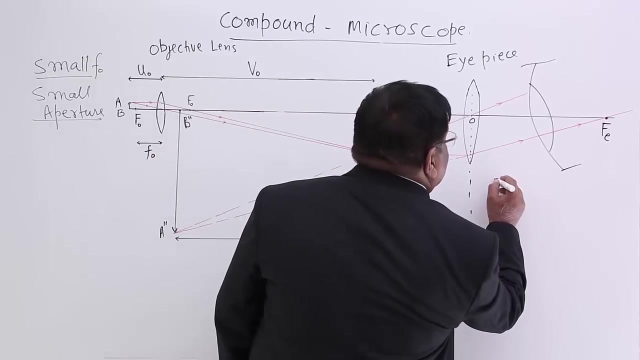 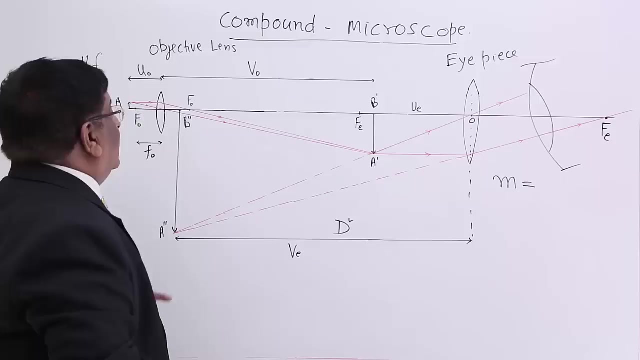 it has become. This is wonder of compound microscope. Now first let us do the calculations. You have understood how these things are placed before the microscope: microscope, and the image is very, very large compared to object. How much is the magnification? The answer is: magnification is size of image divided by size of object, The final image. 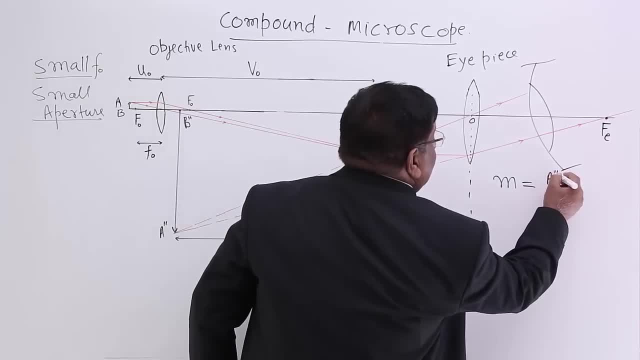 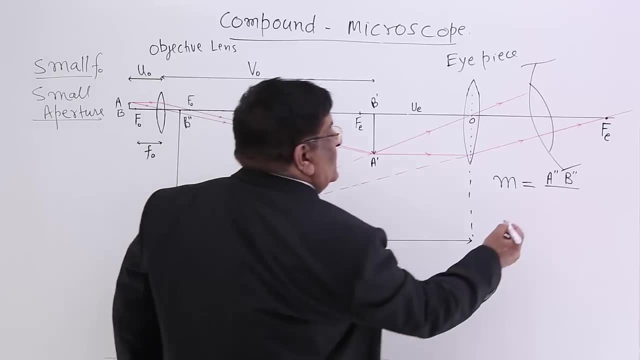 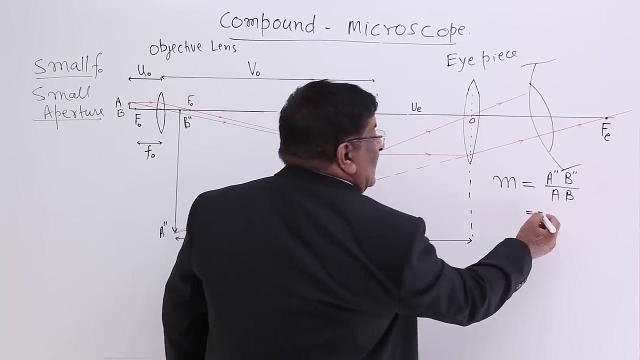 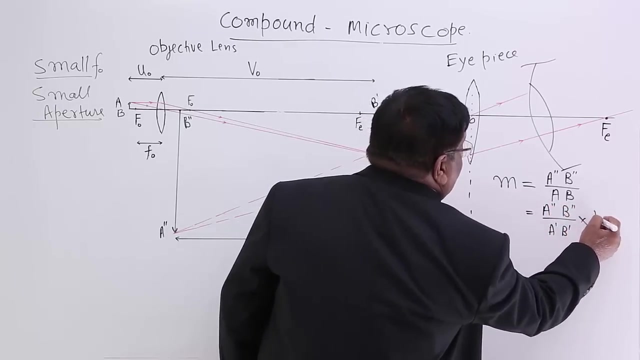 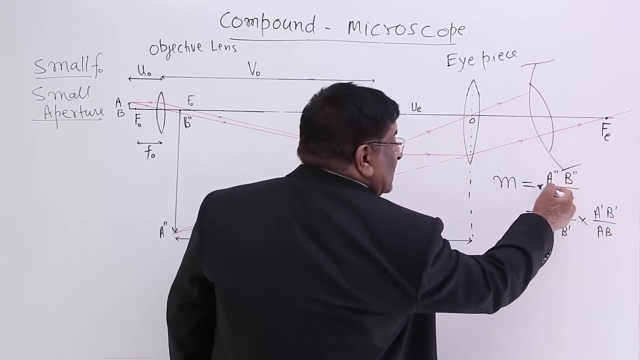 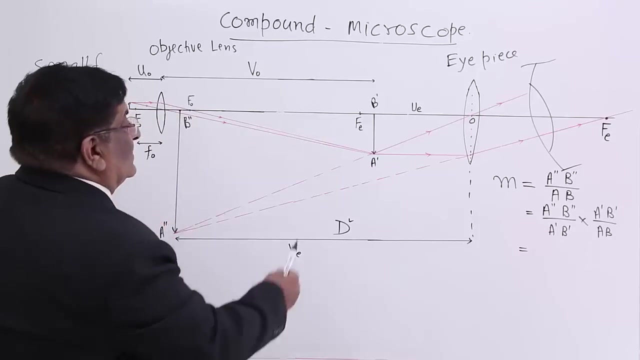 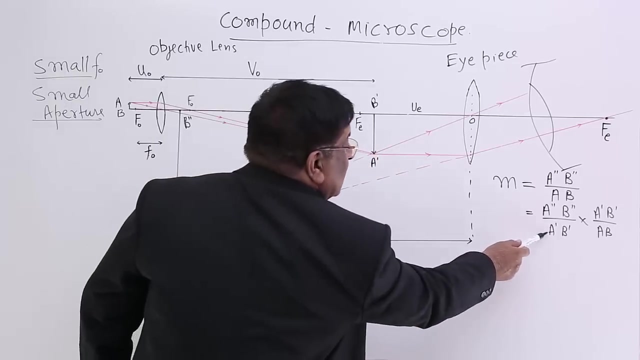 we are seeing is a double dash, b double dash. The original object is a, b. This I can write as a double dash, b double dash divided by a dash b dash into a dash b dash divided by a b. So So this expression is divided by A dash B dash multiplied by A dash B dash. Why This? C? A double dash, B, double dash upon A dash B dash. What is this? This is image, this is object. for this lens, For this lens, this is object. this is image, Object, image. 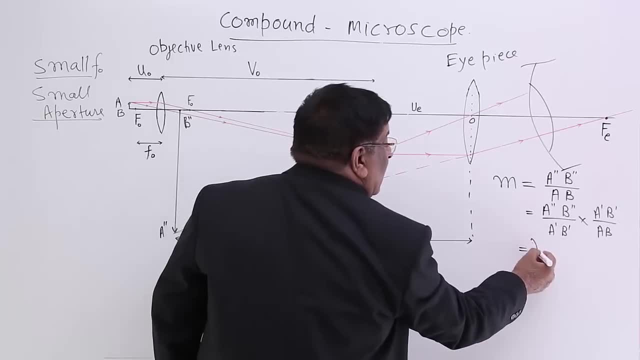 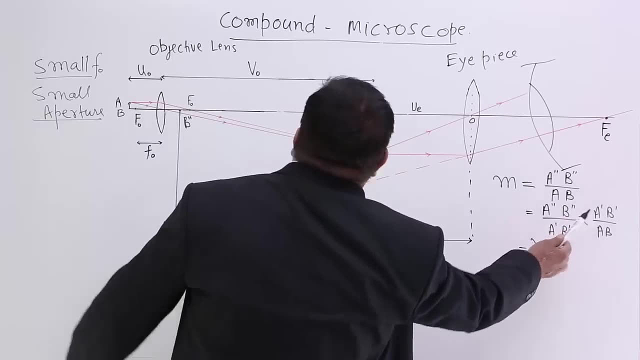 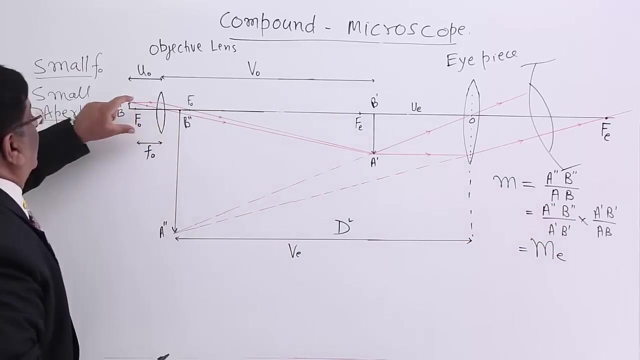 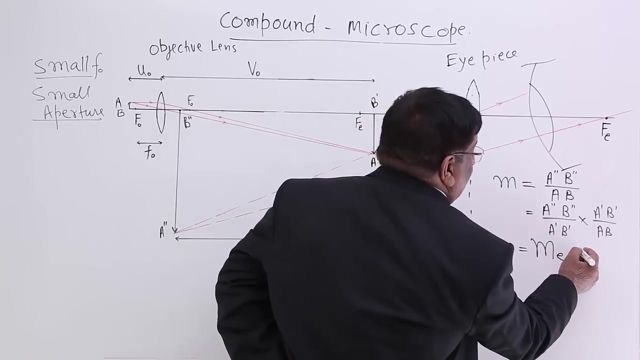 So what is this ratio gives? This gives magnification done by eyepiece. Well then, what is this Image? this lens has made image A dash, B dash. This lens has object A, B, A B, So A dash, B dash upon A B. this represent what Magnification by objective? 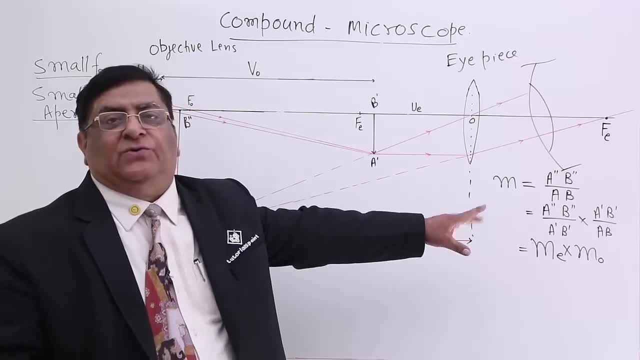 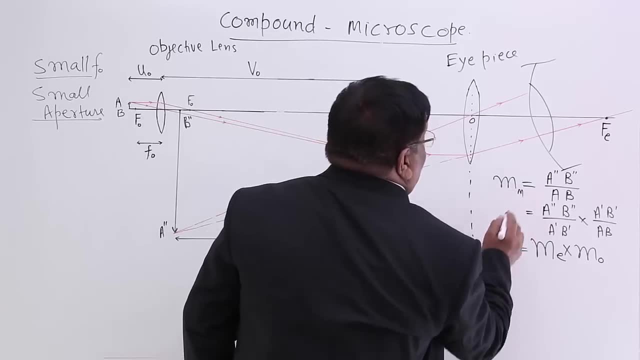 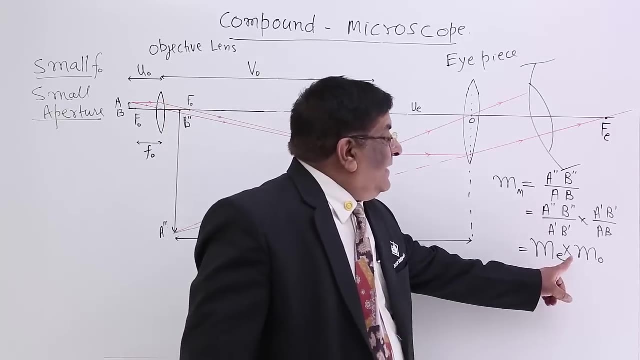 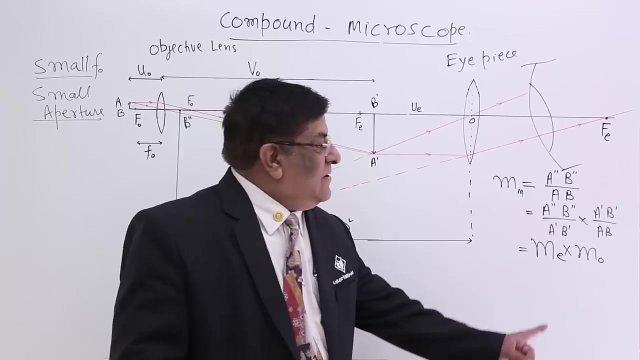 So this is the ratio. So this is the ratio. So this is magnification by eyepiece into magnification by objective. This is magnification by compound microscope. So this is the magnification Multiplication of the two magnifications. Now do we have expressions for this? Yes, For eyepiece magnification. we have done it in the previous lecture. 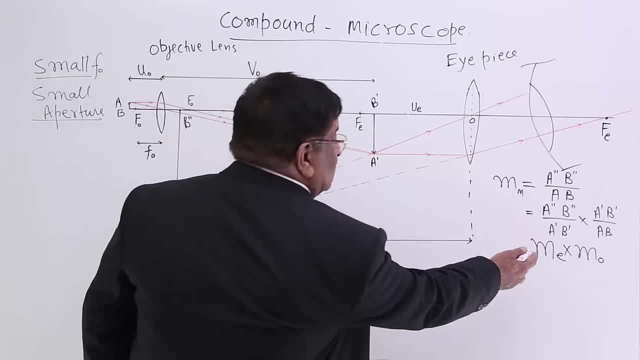 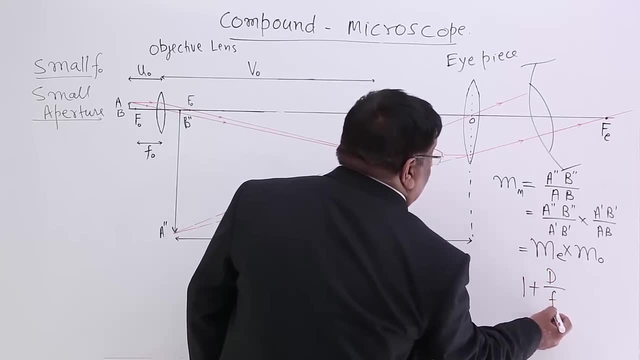 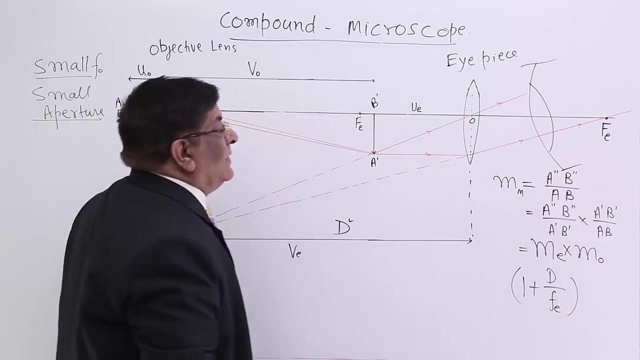 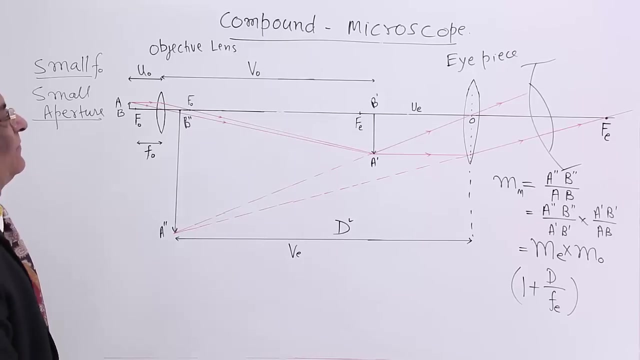 And what is that? For distinct vision, it is 1 plus D upon F, D upon F. Who is F? This lens and this is eyepiece M? O magnification done by this? How much is the magnification done by this? This is a very simple formula: V objective divided by U objective. 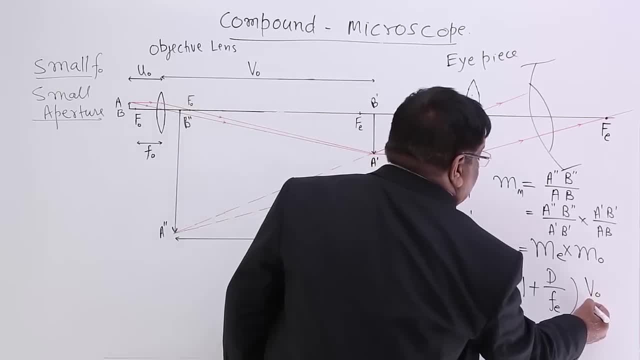 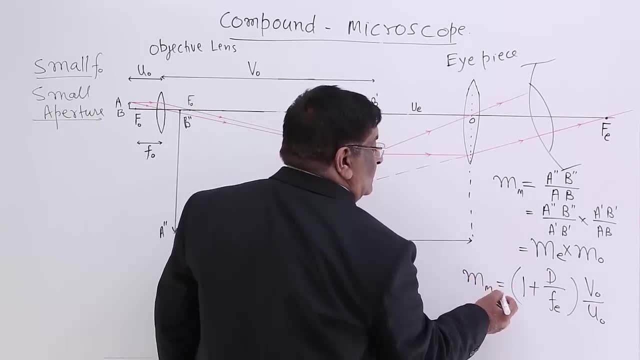 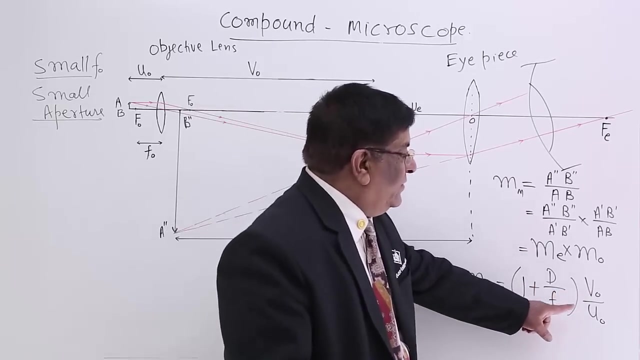 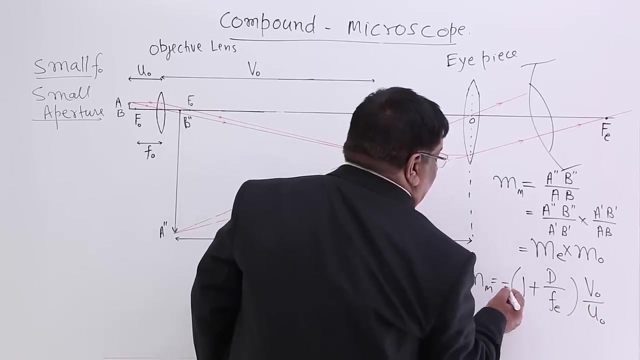 So I write it: V objective divided by U objective. This is magnification, That's all. So this is the formula. And there is one thing: because I am putting these values and U is negative, So this will be minus U dash, and that minus will appear here. 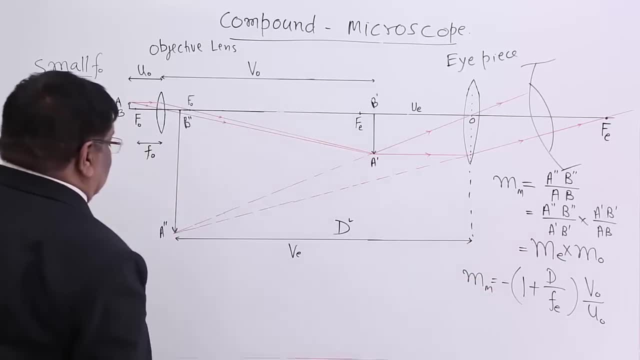 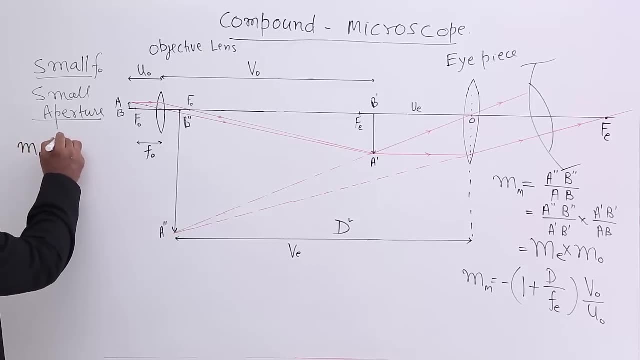 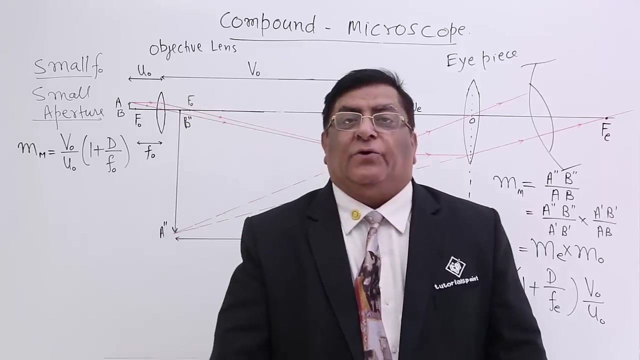 Now, if I write it straight, then this will be: magnification of the compound microscope is equal to V objective upon U objective and 1 plus D upon FO. This is for which setting. This is for distinct vision setting. Now there is another thing Still. we could not find many results. We have calculated: 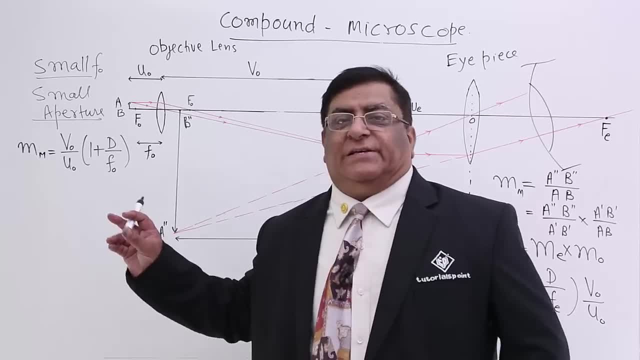 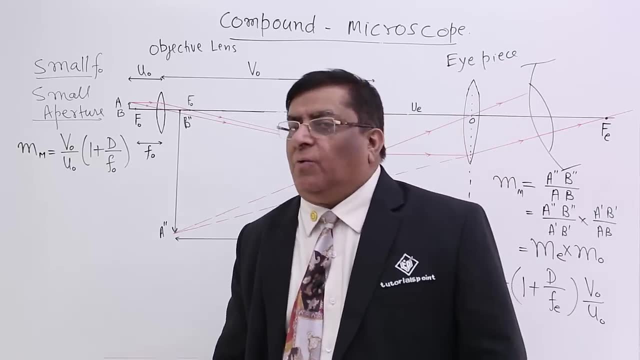 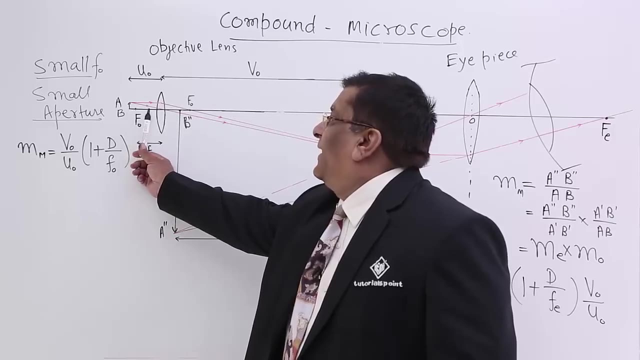 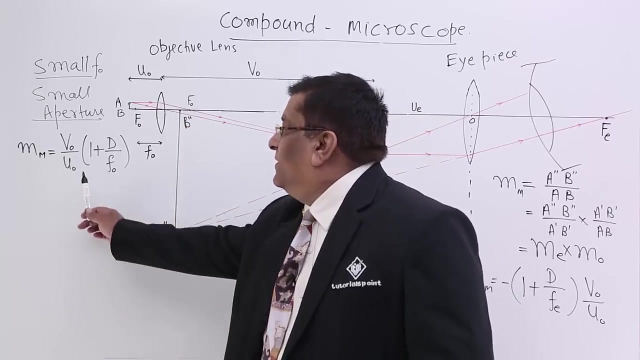 What is the effect of focal length of objective lens? here We do not have it, So we go for certain approximations. What is that approximation For this lens? FO is very close to object. FO is very close to objective, U objective. So for an approximation we can replace this with FO number 1.. Number 2, what? 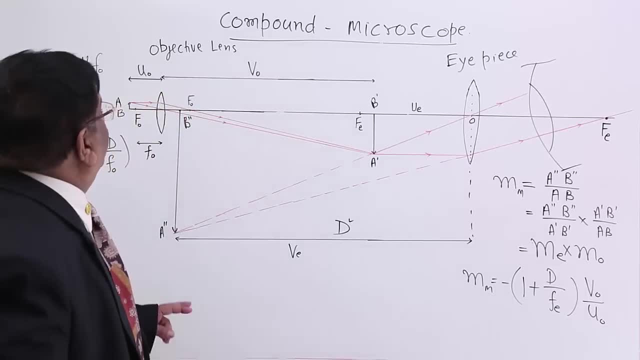 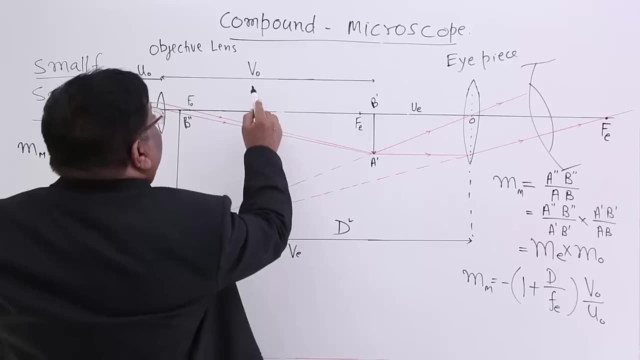 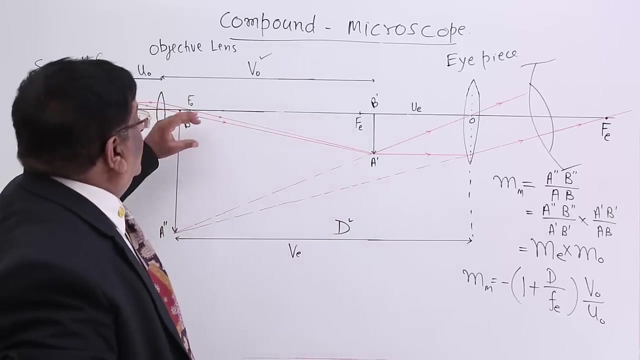 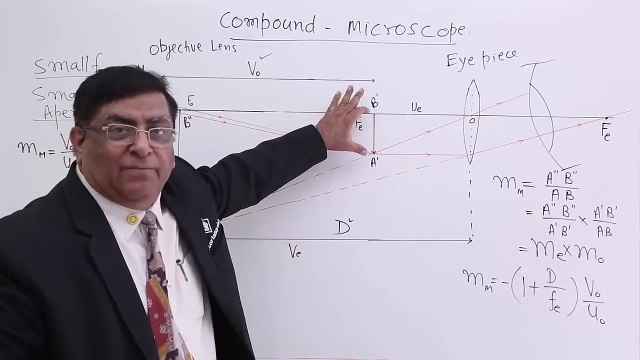 is length of the microscope. Length of the microscope is from this lens to this lens and most of this length is covered by VO. So more length is available, more will be VO, because more is the VO, more will be this magnification. This magnification is a real. 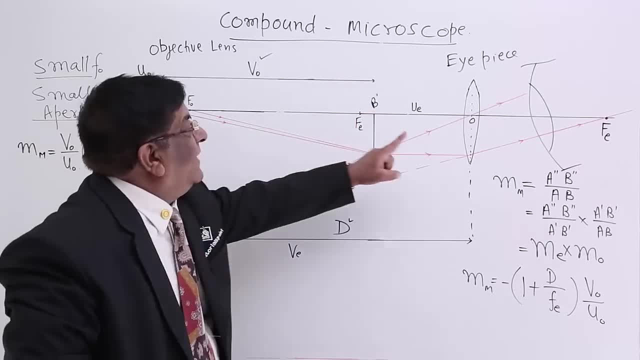 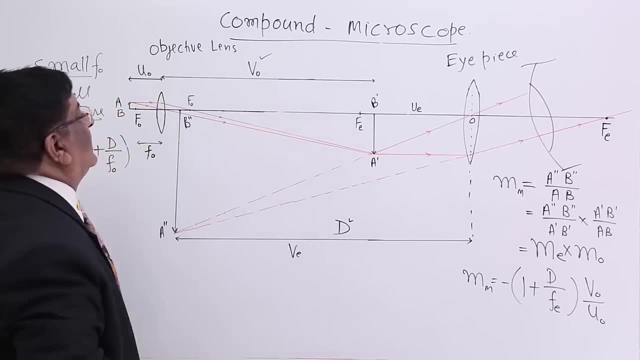 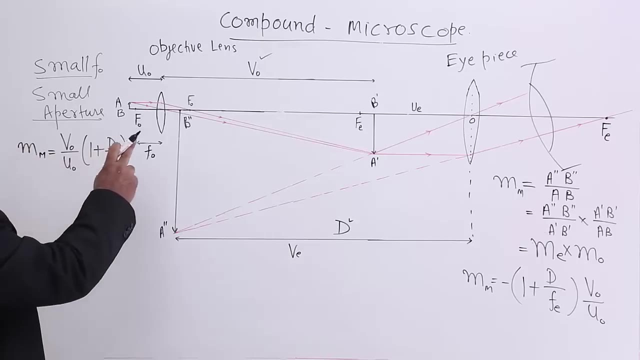 magnification and it has to be within the microscope. So more is the length, more is the VO. So we can take roughly that VO is very close to, not very close to VO is very roughly equal to length of the microscope. In that case this will be: 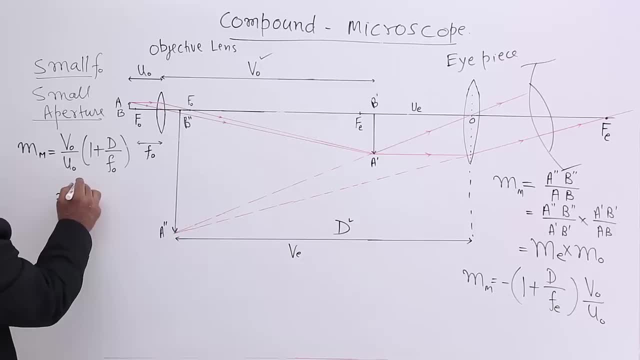 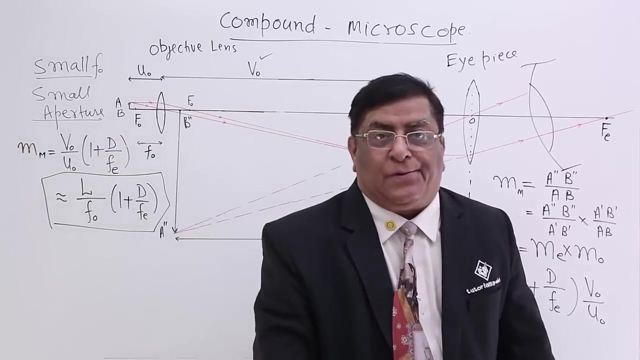 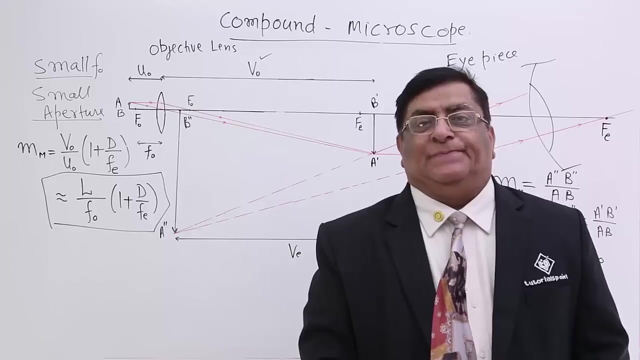 approximately equal to length of the microscope divided by FObjective 1 plus D upon O FIPs. This is our formula for magnification: approximate formula, not the exact formula. This is the exact formula. If we want a setting which is for parallel rays, for relaxed eyes, then I will slide. 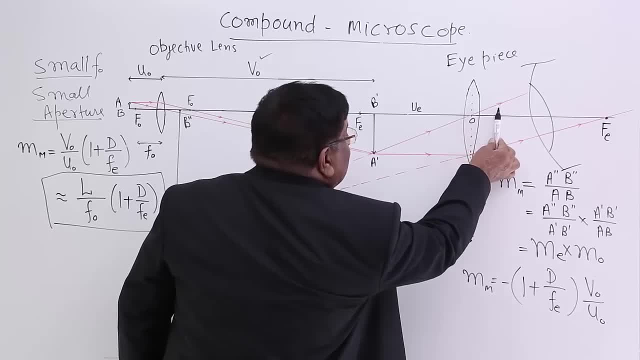 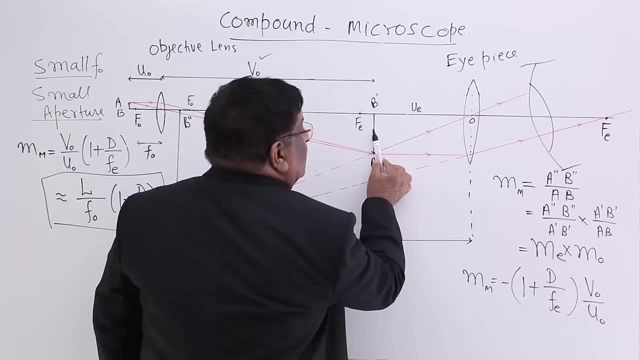 this this way: If I slide it a little here, then this F will come here When this will be lying on the focus of it. then these rays, these two rays, will become parallel, because the object is placed on the relative basis and the distance between the rays are kept. 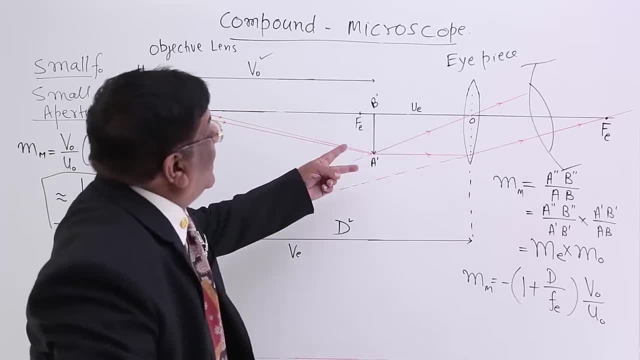 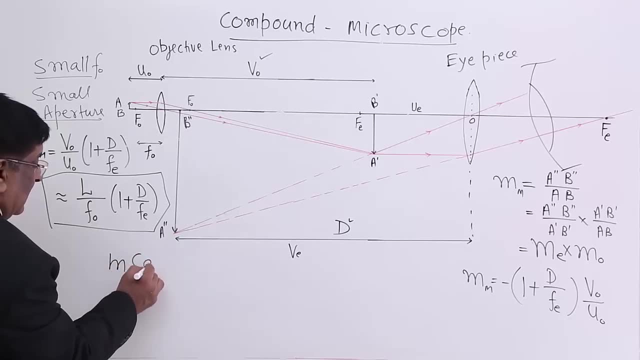 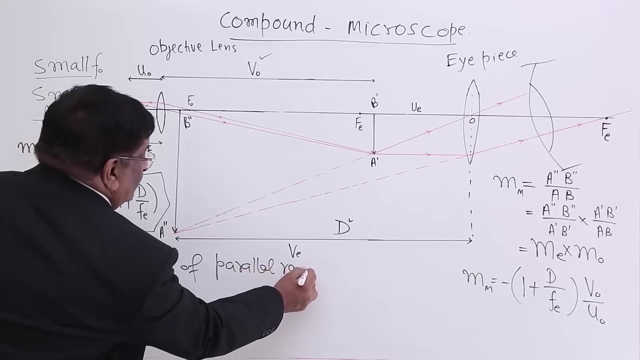 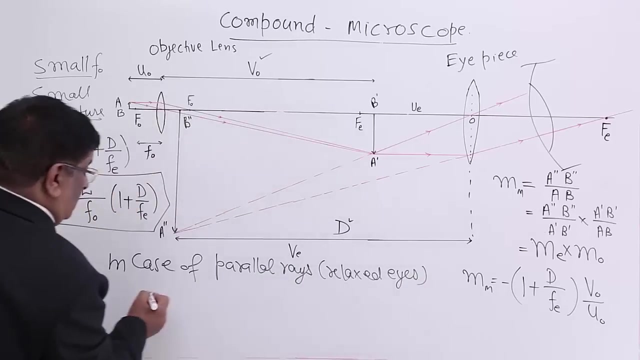 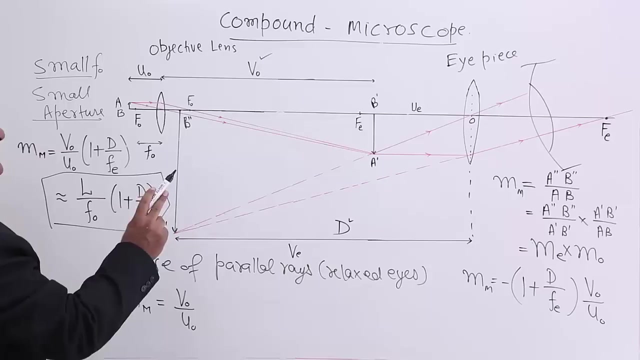 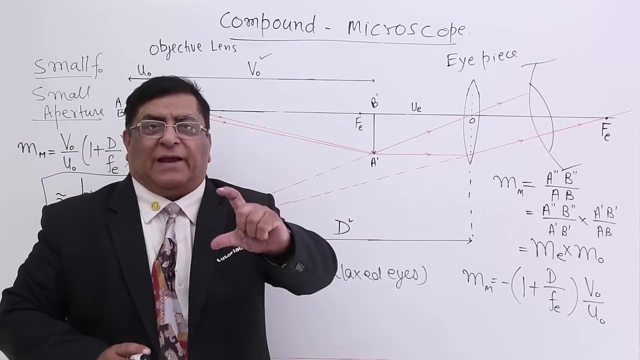 parallel focus, Then we will get parallel rays coming to the eyes and in that case, in case of parallel rays, relaxed eyes, magnification by microscope is equal to Vo upon Uo multiplied by d upon Fe. because you remember, for that setting, for relaxed eye setting, what is the magnification? 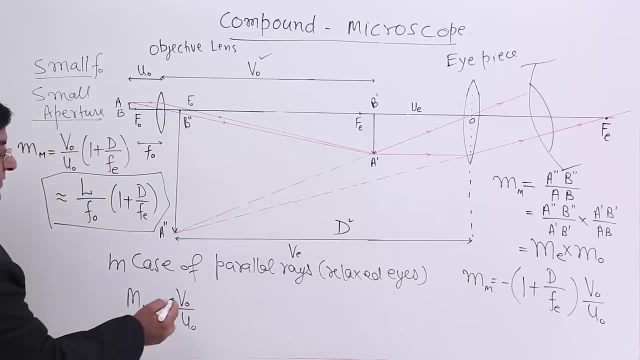 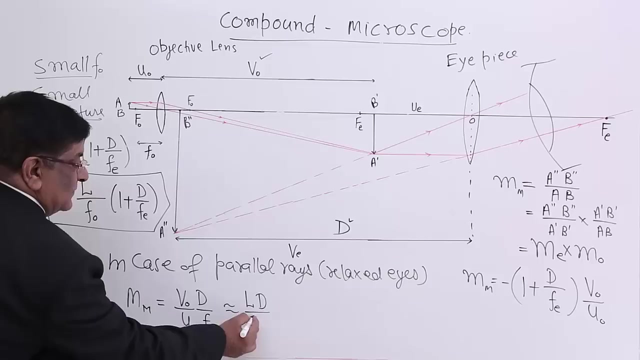 d upon F, So we use here d upon Fe, and very roughly. this is equal to L length of the microscope, d, which is a constant. this is focal length of objective and this is focal length of eyepiece. This is an expression which helps us to understand the nature of microscope. 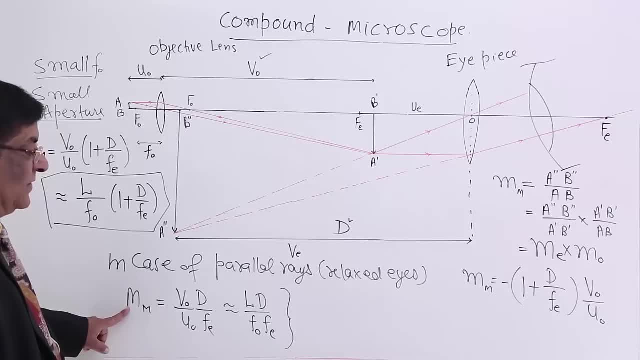 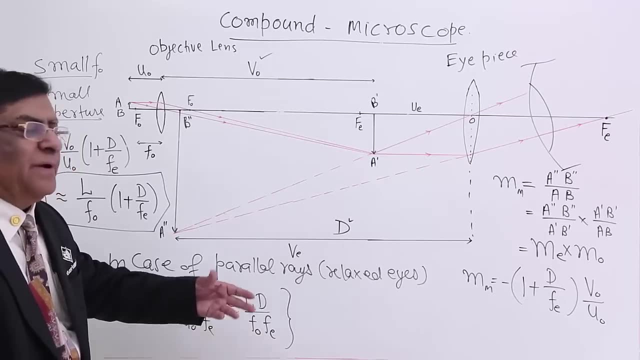 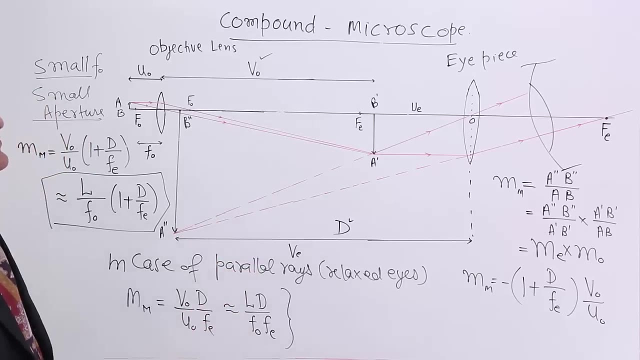 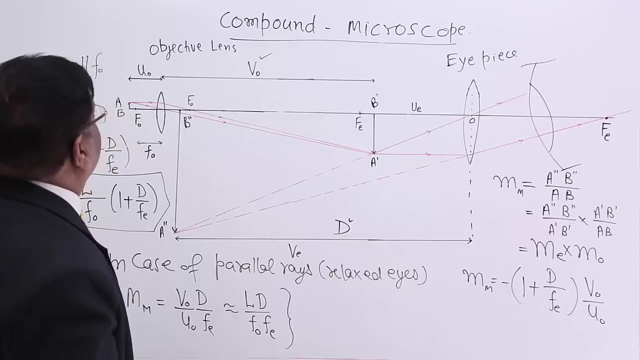 If we want a large magnification, Fo should be small as well as Fe should be small. Yes, the length may be large, but only length won't do Fo and Fe. they should be small Plus what should be the length Length. we can have this Vo plus this, so no expression for that. 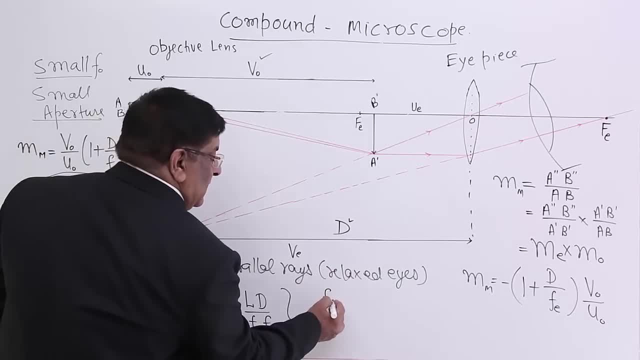 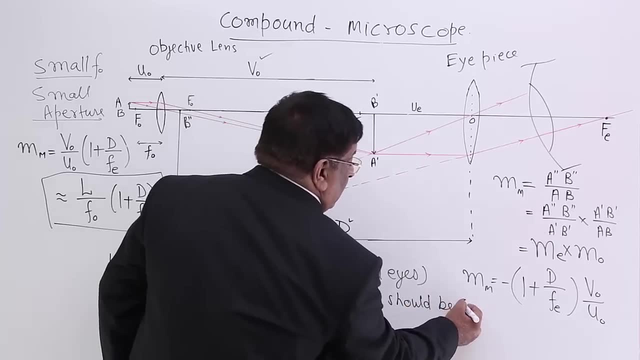 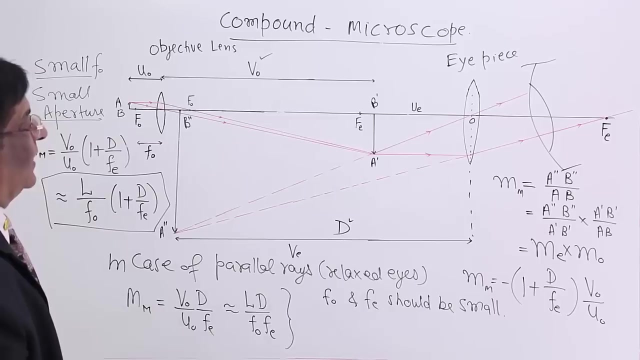 So this we should understand. Fo and Fe should be small, gotten tasty joined. Okay, so this is simple microscope and so much is the magnification. so there are two expressions, three expressions: one, one, two, two. 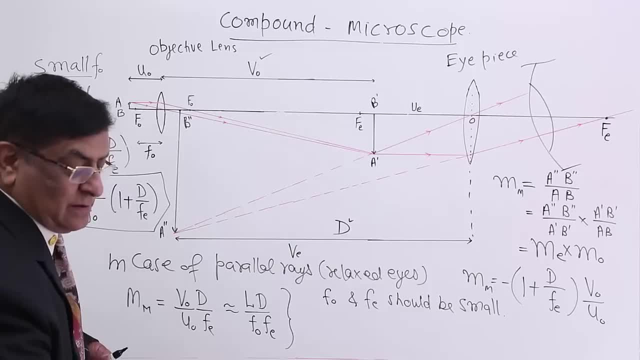 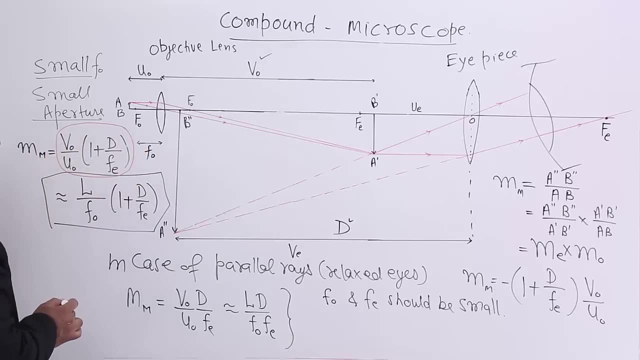 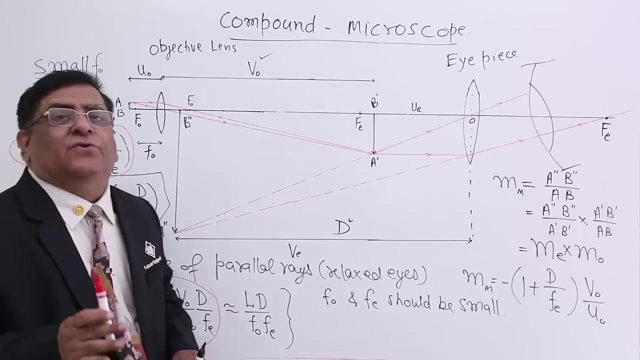 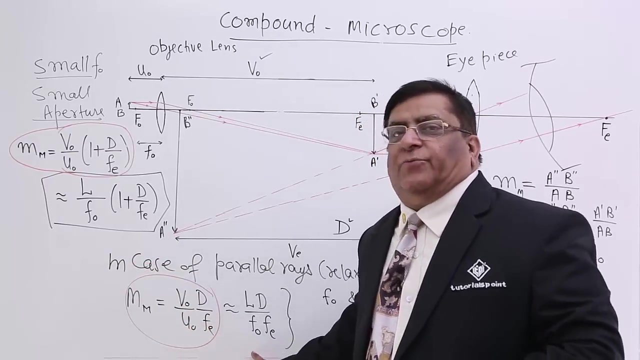 is this expression. whenever we are doing calculation in the numericals, we will do this expression and we will use this expression. please remember, do not use these expressions because these are very approximate, unless you have to give a rough idea and you have to study what is the effect of focal length of objective and focal length of eyepiece.